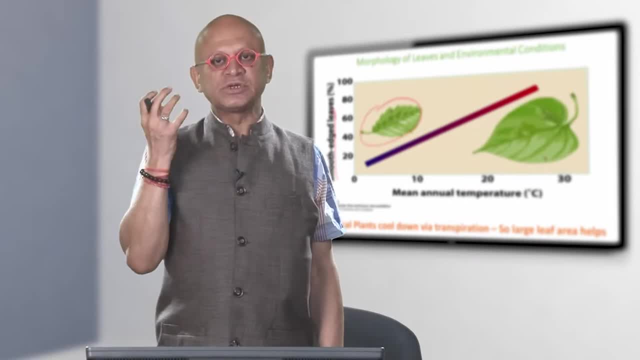 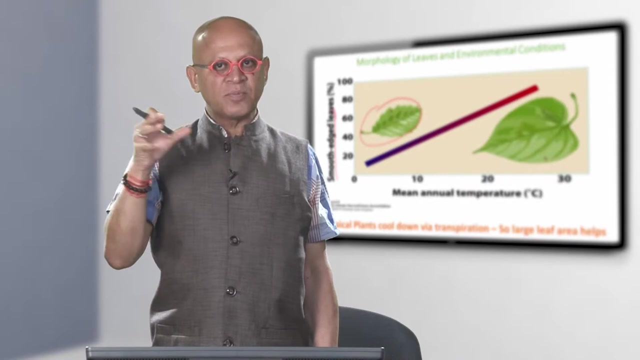 supposed to capture sunlight, capture carbon dioxide, And when the stomata opens, they are supposed to open long enough so that not too much of the water that has been supplied by the roots is going to get lost to the atmosphere. So this optimization, obviously, is going to 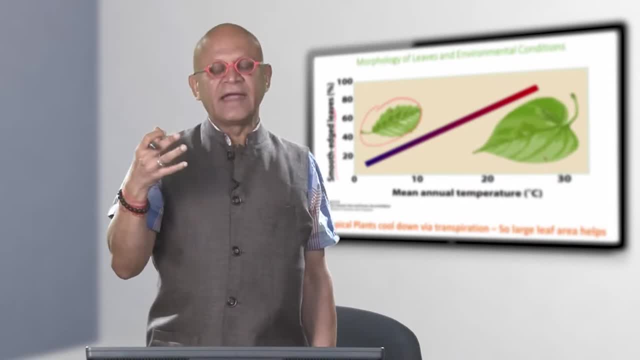 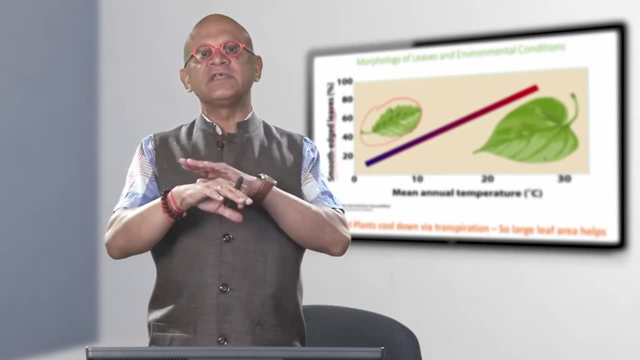 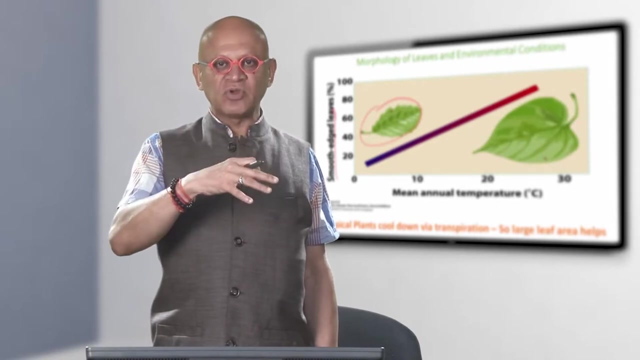 depend on the temperature, Plus. at very high temperatures the leaves themselves have to cool down, So they do it through, basically like a respiration or sweating. That's called transpiration. So there is evapotranspiration, evaporation and transpiration by the plants. 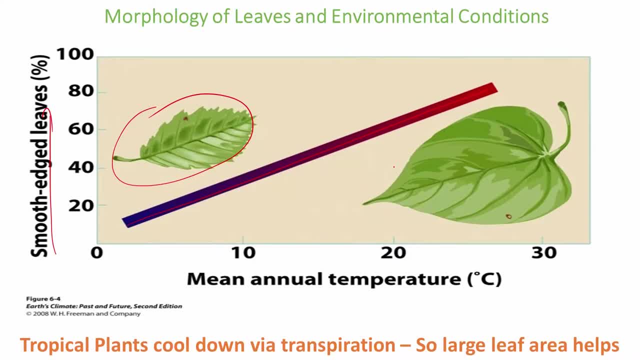 So that determines the size of the leaf. And as the temperature increases, they want to sweat more, So they increase their temperature. So that determines the size of the leaf. And as the temperature increases, they want to sweat more, So they increase their. 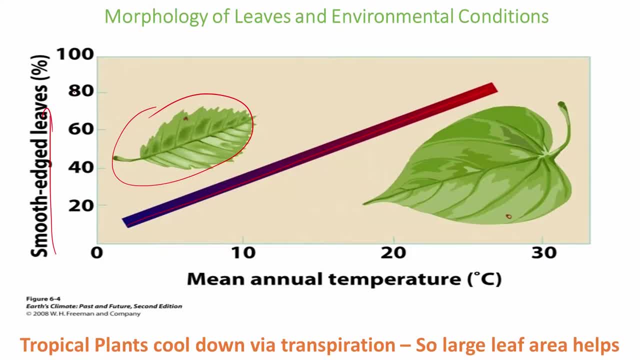 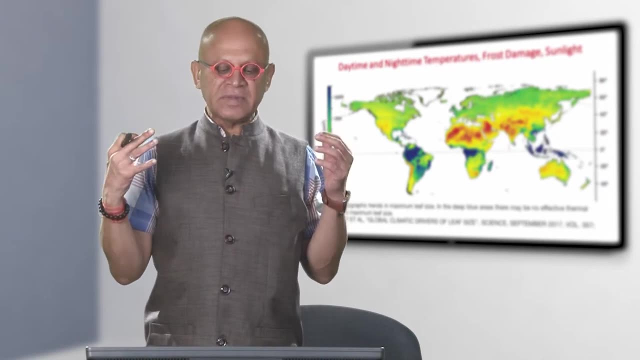 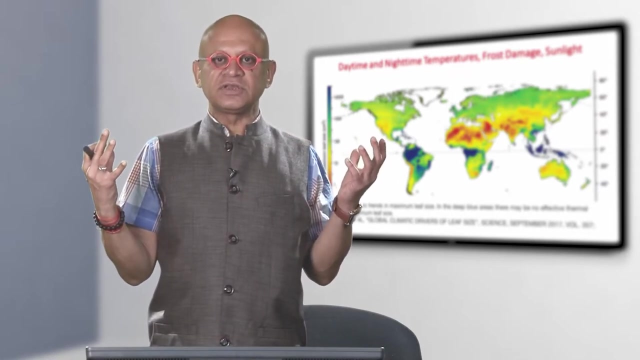 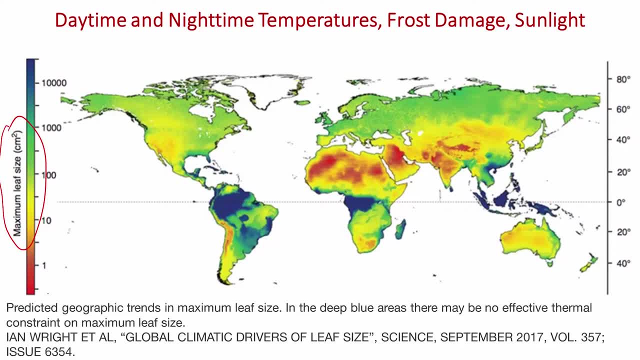 maximum leaf size in cm2 going from close to 0 to more than 10,000 cm2.. So you can see that the map is showing there are regions, like the rainforests of Amazon, Central Africa, Indonesia, the so-called maritime continents and so on, where there is essentially 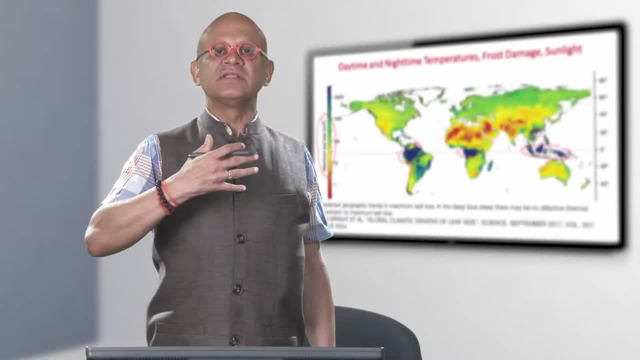 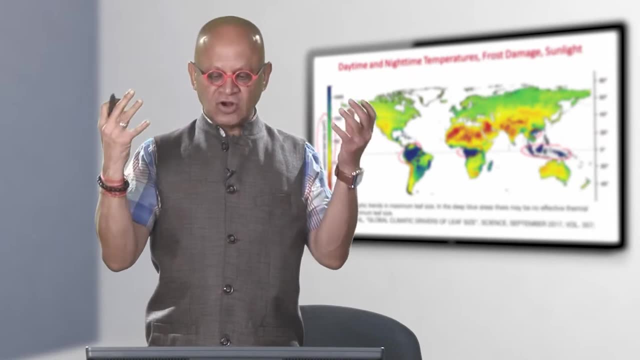 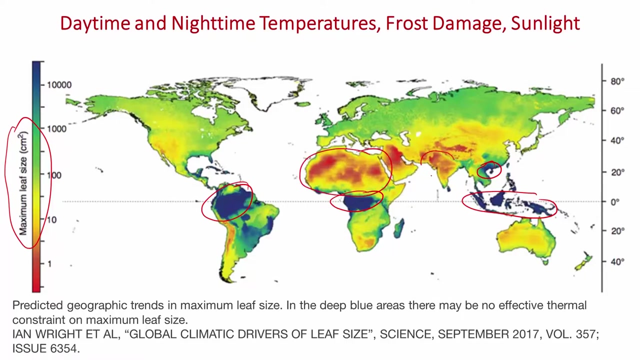 no impact of temperature on the leaf size. That means the humidity temperature. the difference between daytime and nighttime temperatures are pretty minimal, so the leaves are not showing any impact, whereas if you go over the desert regions or even over the monsoon regions, over India and so on, the leaf size